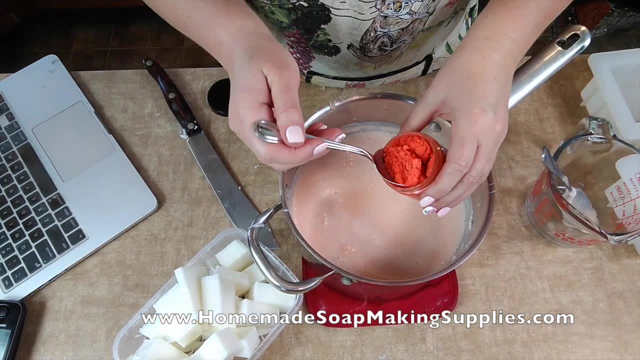 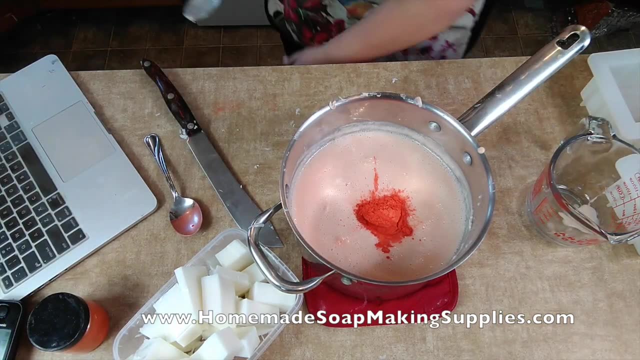 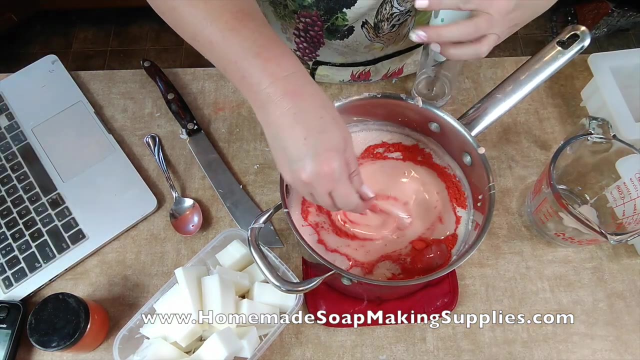 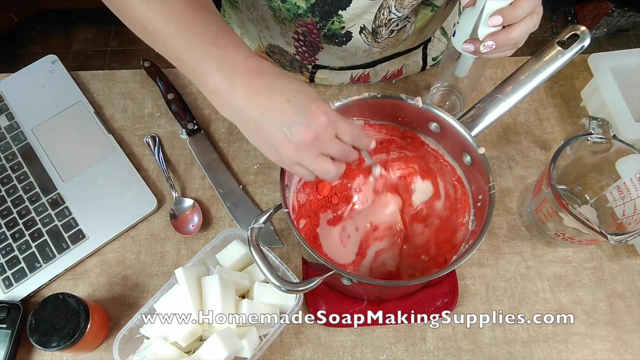 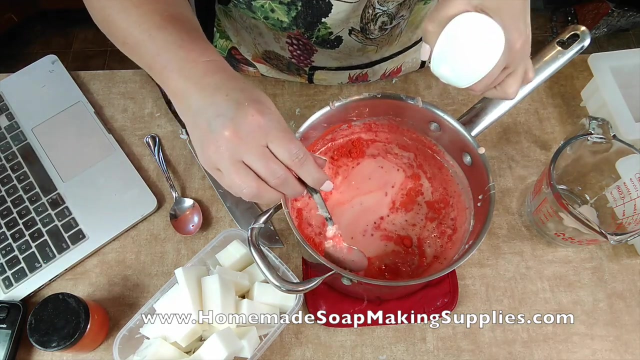 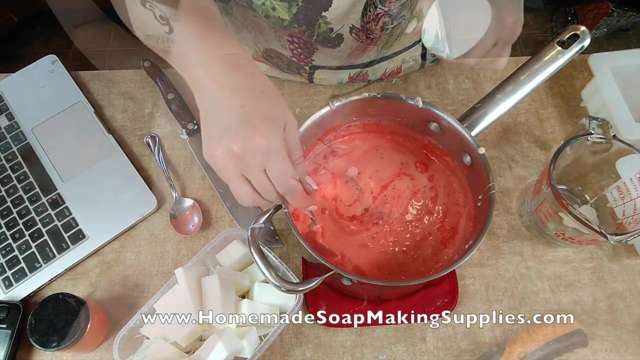 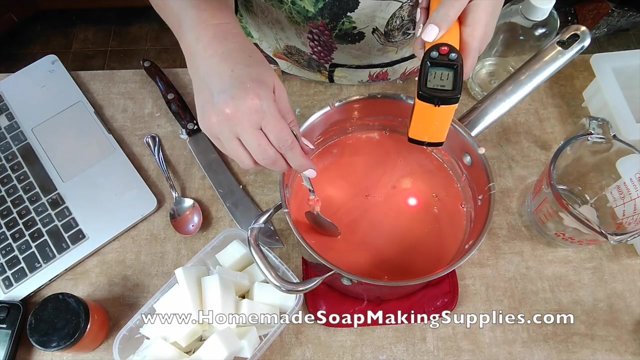 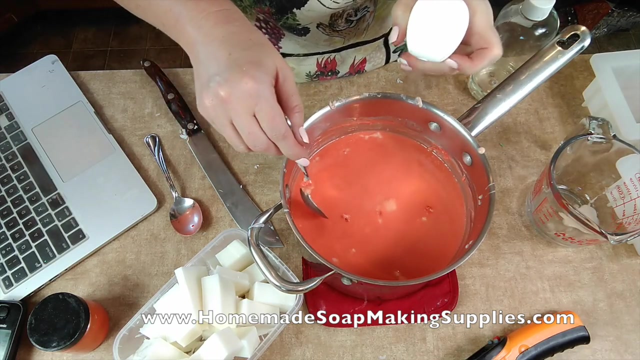 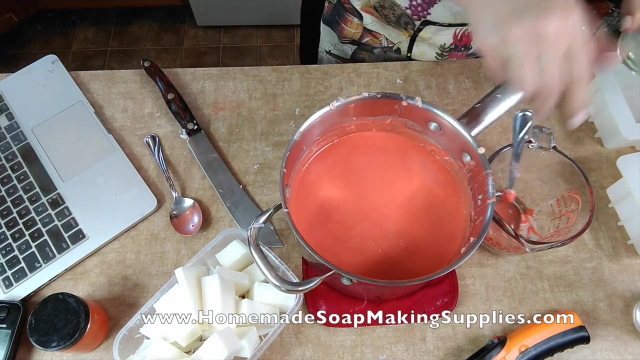 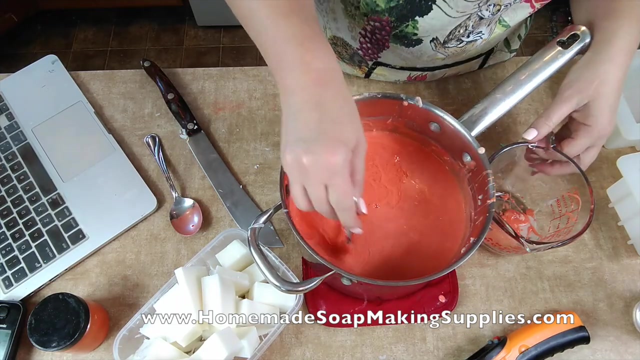 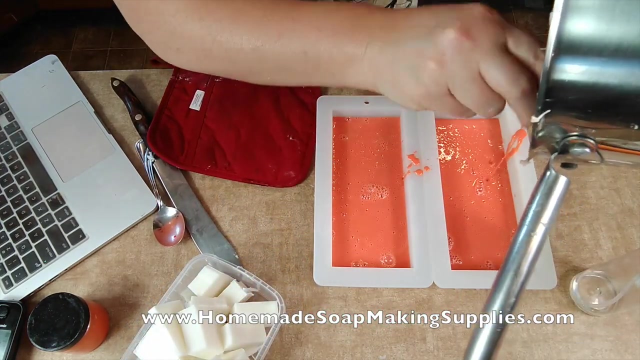 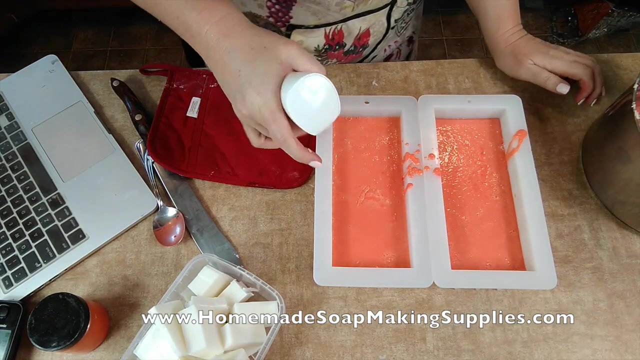 Put in the color Spray, alcohol on it and it breaks up the mica clumps. Okay, so the temperature is 170 for putting our fragrance oil in, And we're almost there. Oh, that smells really good. Okay, so I'm. 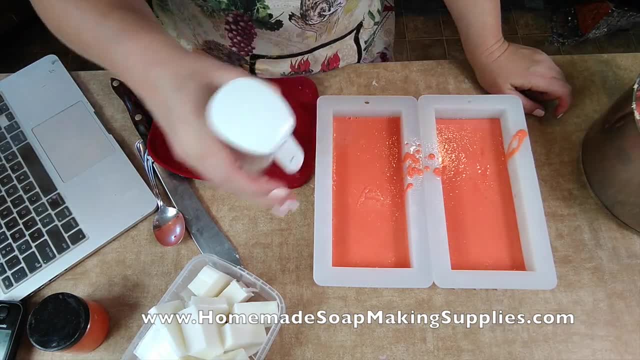 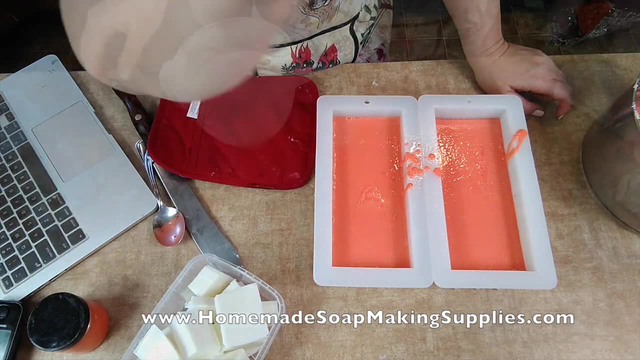 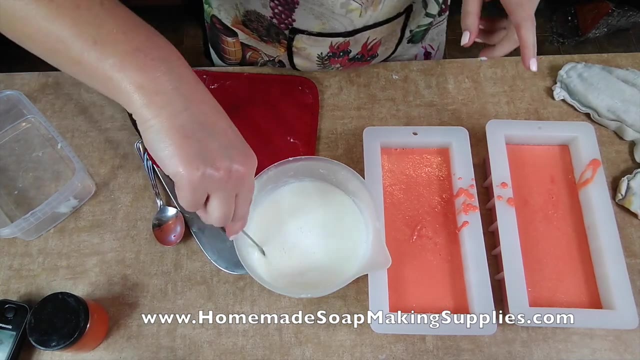 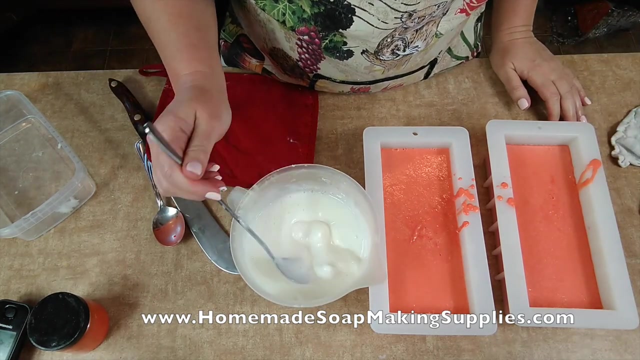 spraying this to break out the little bubbles. I'm going to let this set up and then we're going to melt our white and put it on top. Alright, so I have my top not quite melted. Stir it around just a little bit until it melts. 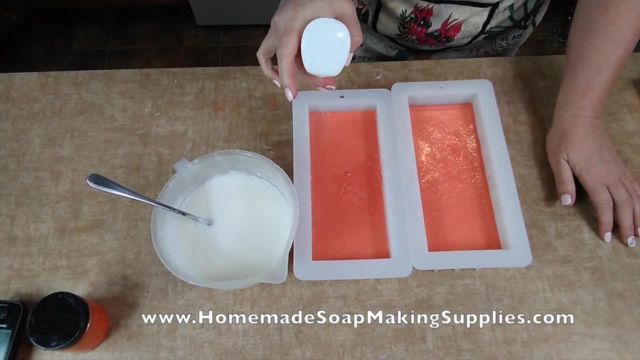 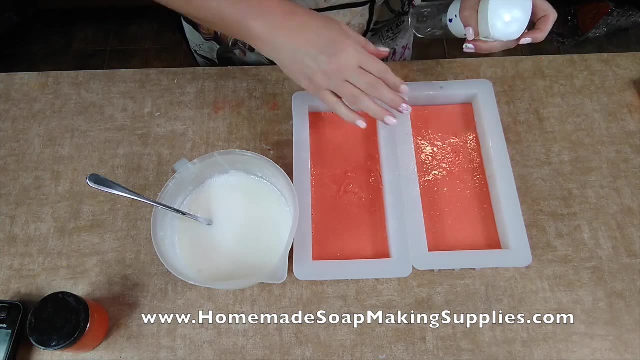 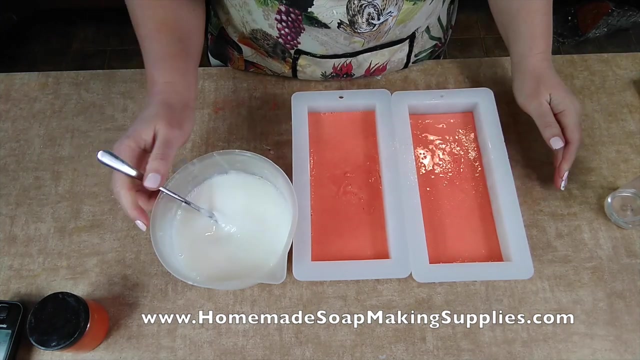 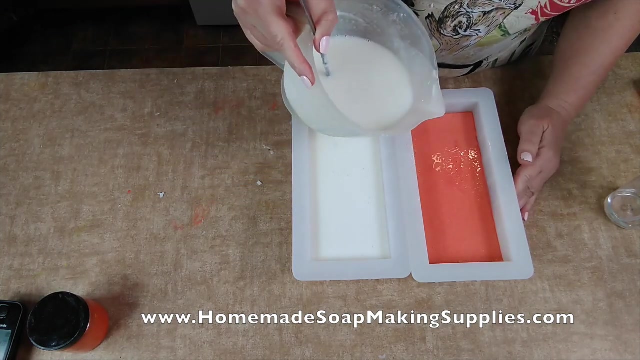 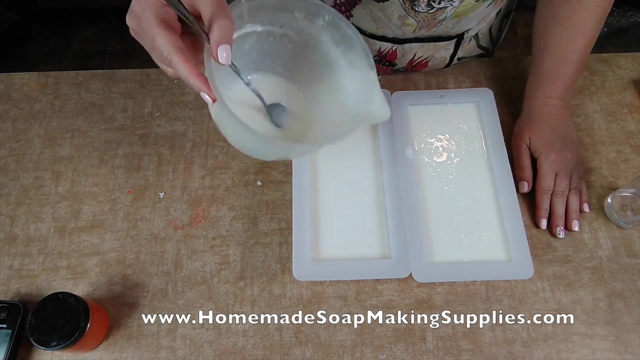 Okay, then you're going to liberally- I'm almost out of rubbing alcohol, but you're going to liberally- spray your first layer with rubbing alcohol So that the second melt and pour will adhere to the top. Okay, And there we go.